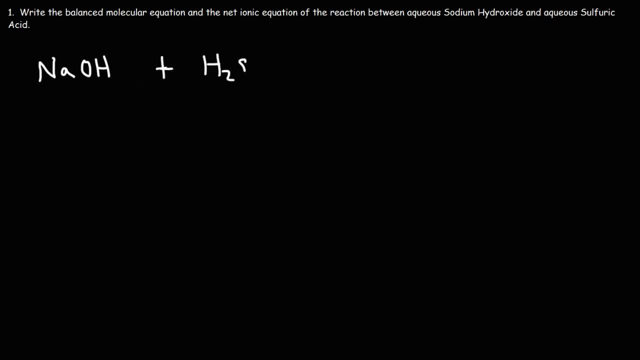 sulfuric acid is H2SO4.. Now both of these are in the aqueous phase, which means that they are dissolved in water. Now this is what is known as an acid-base neutralization reaction. H2SO4 is a strong acid. A solution with that compound has a very low pH. Sodium hydroxide. 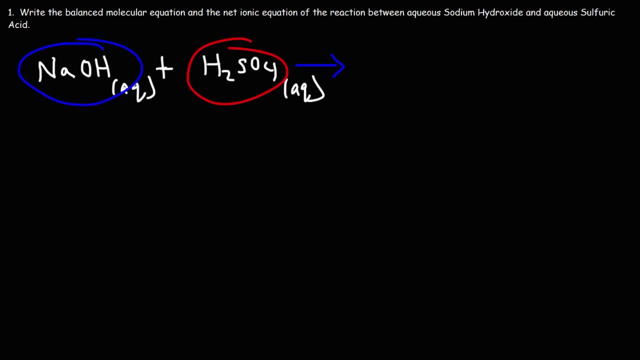 is a strong base A solution could be a very strong base A solution could be a very strong base A solution contained in NaOH has a very high pH. When you mix these two together in equal amounts, they will neutralize each other, such that you get salt and water with a pH of around 7.. 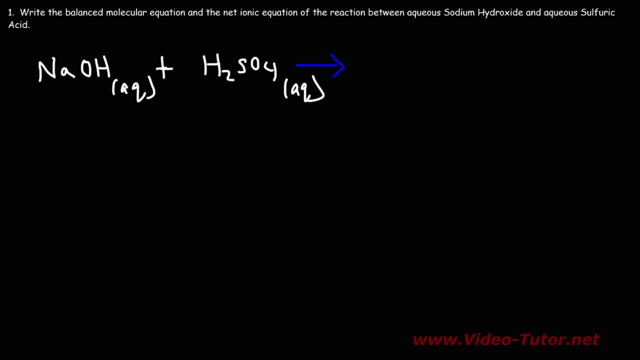 Now let's talk about the products of this reaction. Hydroxide is going to pair up with the H plus ion. When these two get together, they will produce water, And water is in the liquid state. Sodium is going to pair up with sulfate. 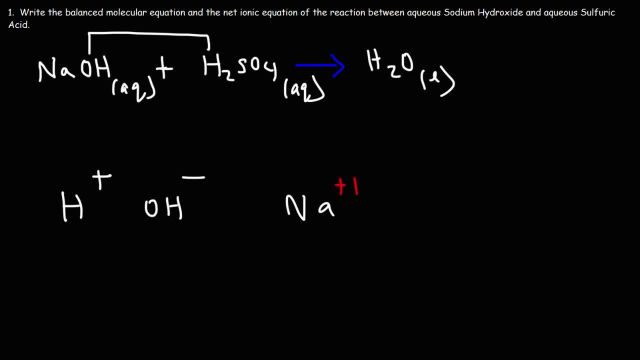 Sodium has a plus one charge. Sulfate has a two minus charge. So in order to balance the charges, you need to use two sodium ions and one sulfate ion. So the chemical formula for sodium sulfate is Na2SO4.. And sodium sulfate is soluble, so this is going to be aqueous. 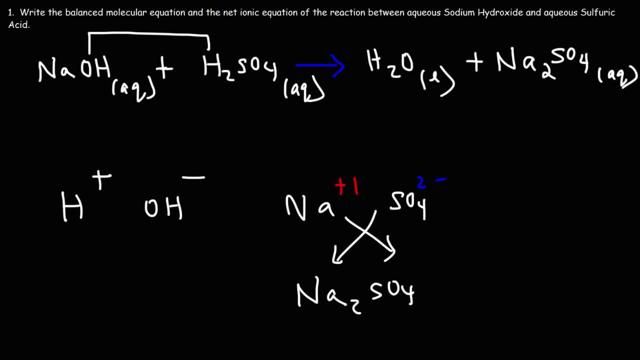 Now that we have our molecular equation, the next step is to balance it. So notice that we have two sodium ions on the right side. We need to put a two in front of NaOH. We have one SO4 unit on both sides, so that's good. 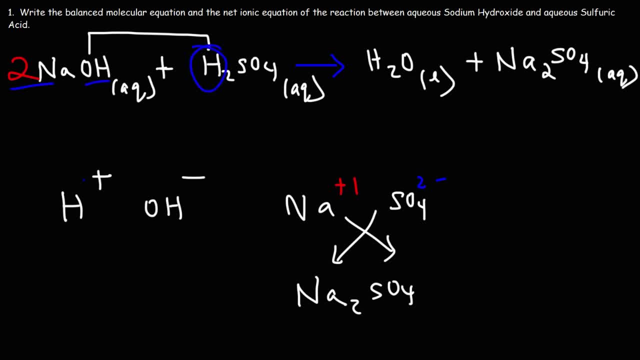 And here we have two hydroxide ions and two hydrogen ions. When you mix two hydrogen ions and two hydroxide ions, you're going to get two water molecules, So we need to put a 2 in front of H2O. 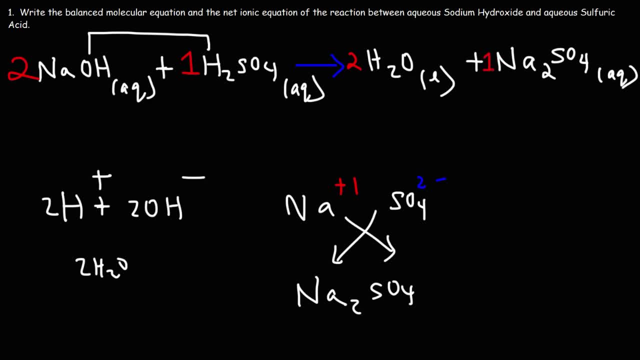 So now the chemical reaction is balanced. We have two sodium ions on both sides, We have a total of four hydrogen atoms. This is two, 2,, this is another 2, and here we have 2 times 2, which is 4.. And we have a total of 6 oxygen. 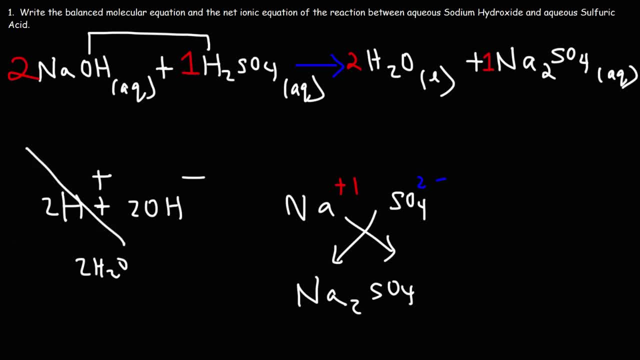 atoms on both sides. So we have a balanced molecular equation. Now, in order to write the net ionic equation, we need to write the total ionic equation first. To do that, everything in the aqueous phase, we're going to separate it into ions, So we're going to break up. 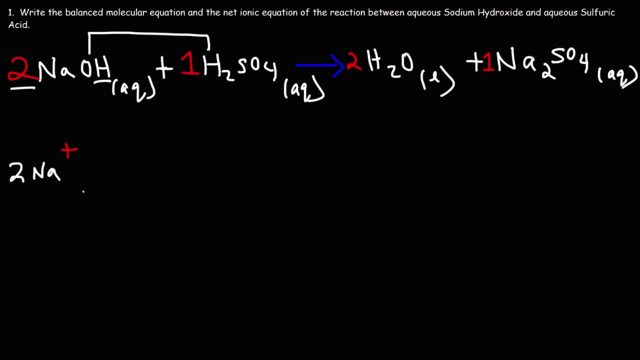 any OH into 2 sodium ions and 2 hydroxide ions. All of these ions are in the aqueous phase, but I'm not going to write aq because I might run out of space. Sulfuric acid is in the aqueous phase, so we can break it up as 2H+ and 1 sulfate ion. Water is in the 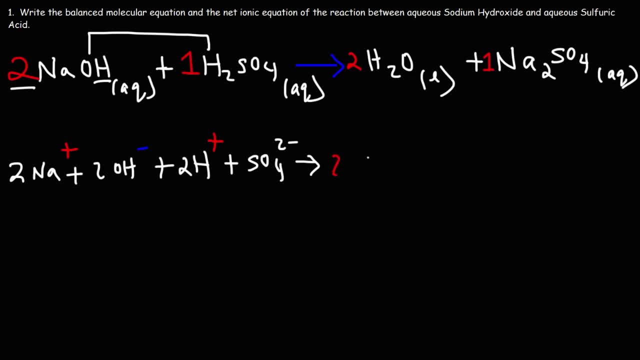 liquid phase. so we're not going to change that. We're going to just separate it into ions and leave it the way it is. Sodium sulfate is in the aqueous phase, so we're going to break that up into 2 sodium ions and 1 sulfate ion. Now, in order to write the net ionic equation, 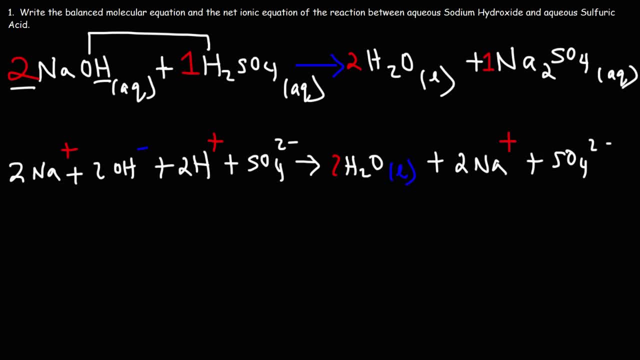 we need to eliminate the spectra ions. The spectra ions are the ones that appear exactly the same on both sides. Thus they can be eliminated, So this includes the sodium ions and also the sulfate ions. Now what we have left over is going to be the net ionic equation: So 2, hydrogen ions. 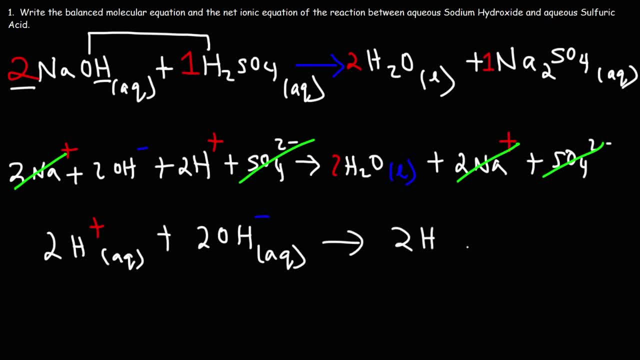 react with 2 hydroxide ions to produce 2 sodium ions. So this is going to be the net ionic equation. So we're going to divide this by 2, and we're going to get the net ionic equation as follows: 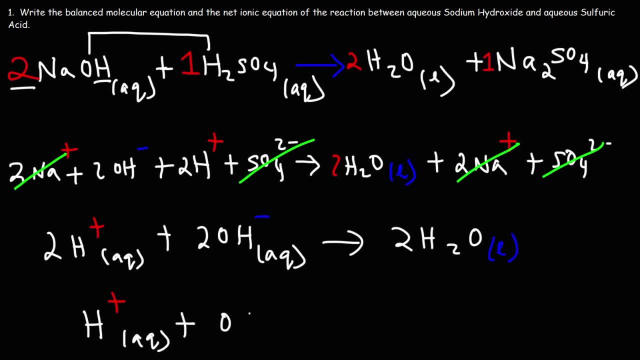 So we have H+ reacting with OH- to generate 1 molecule of H2O. So this, right here, is our net ionic equation, which is typical for an acid-base neutralization reaction. So that's it for this video. Thanks for watching.